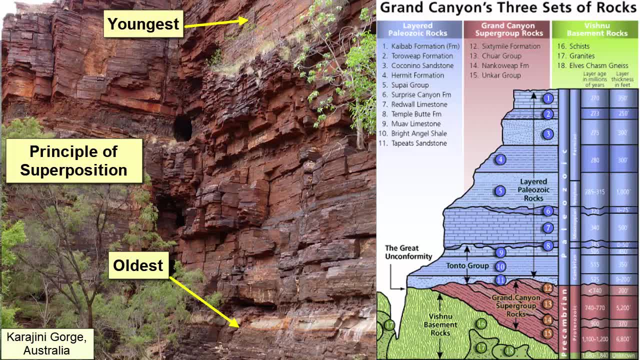 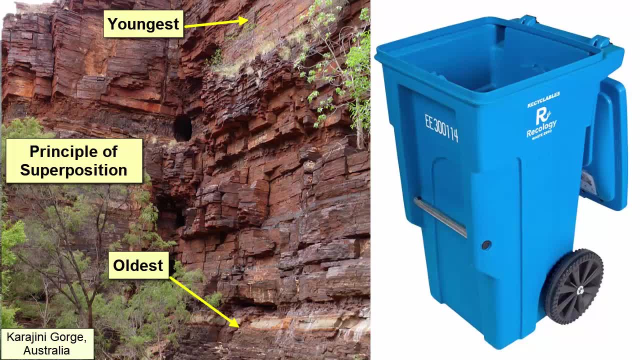 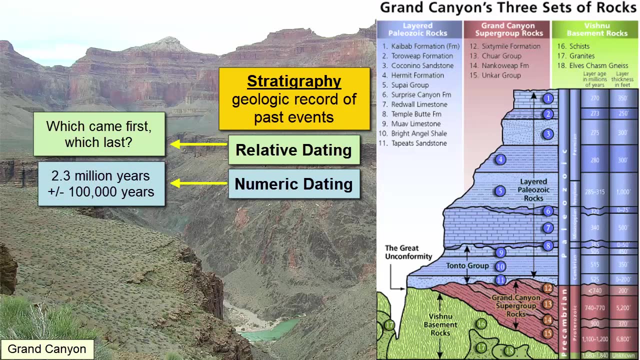 the layers on the bottom will be older than those that deposited on top. A similar process happens with your recycling of newspapers. The oldest newspaper, the one you first threw away, would be on the bottom, the most recent one on the top. Numeric dating applies a variety of techniques to determine a numeric age for a particular. 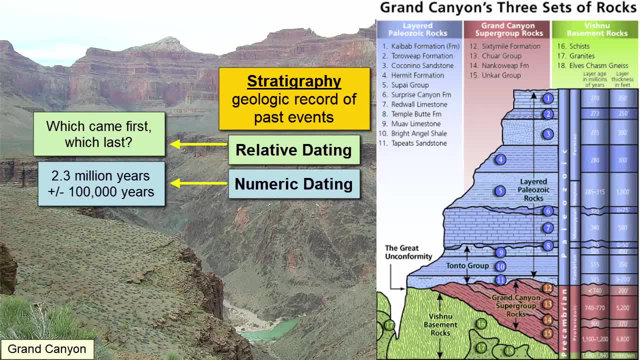 rock layer like 2.3 million years plus or minus 100,000 years. Numeric ages, as you see, have associated errors and can be determined only for rocks that contain the right ingredients, Turns out. most rocks do not have these right ingredients and only some of them can have. 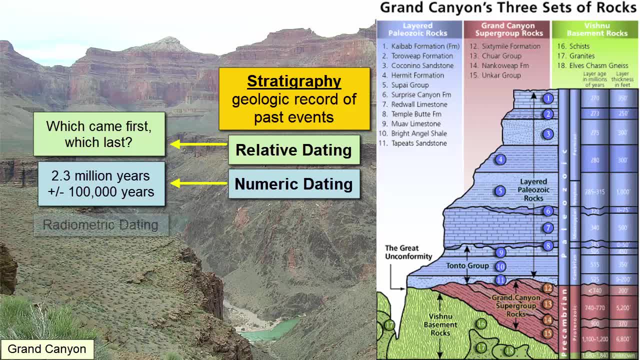 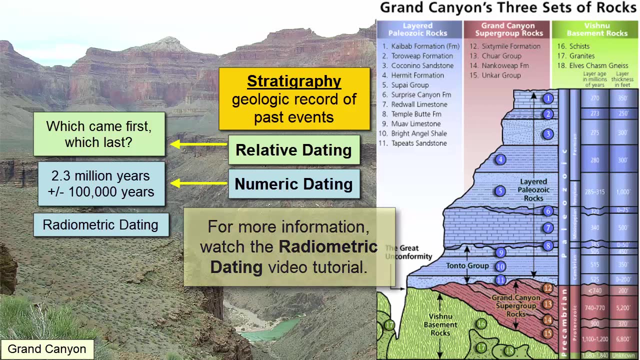 numeric ages associated with them. The most common form of numeric dating is radiometric dating, which uses naturally radioactive elements trapped in rocks to calculate the dates of formation. For more information, watch the video tutorial on radiometric dating. Other types of numeric dating processes include lichenometry- studying the time at which it. 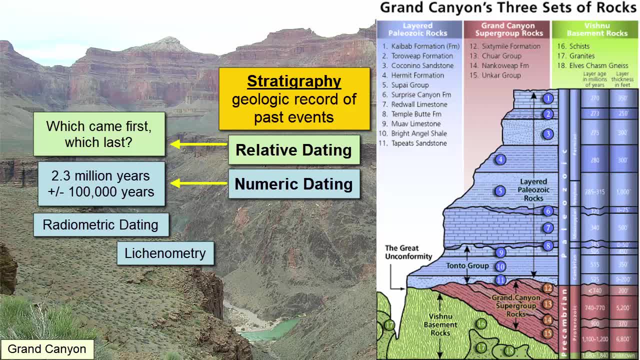 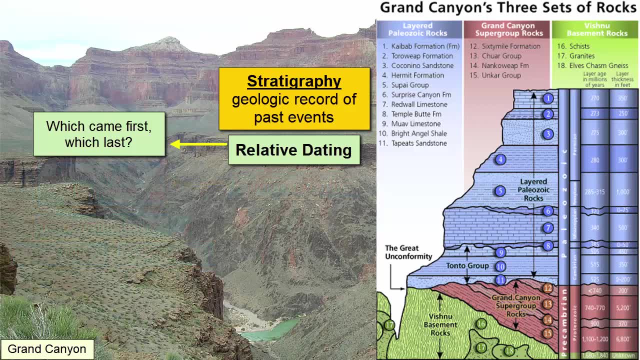 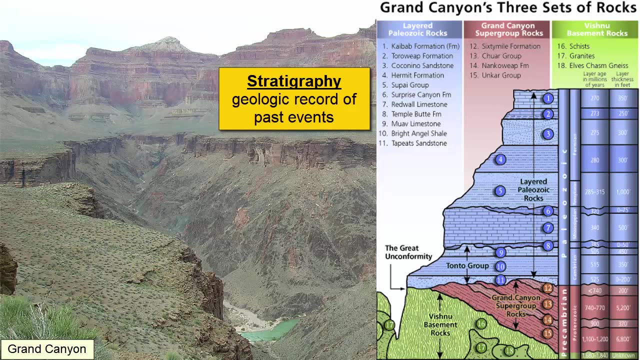 takes for lichen species to grow on a surface of a rock in a particular area, or counting tree rings. For the rest of this video tutorial, we will focus on the following: 1. Relative Dating: To read the rocks and their relative order, to piece together the geologic history of. 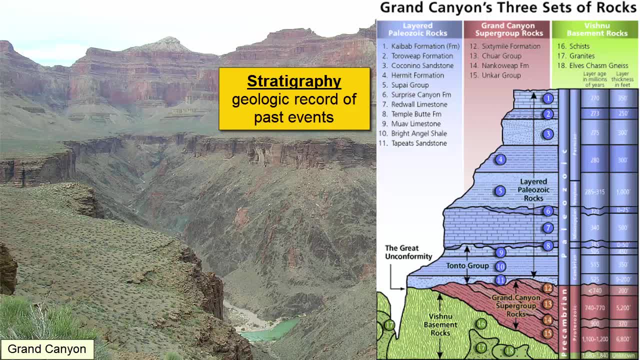 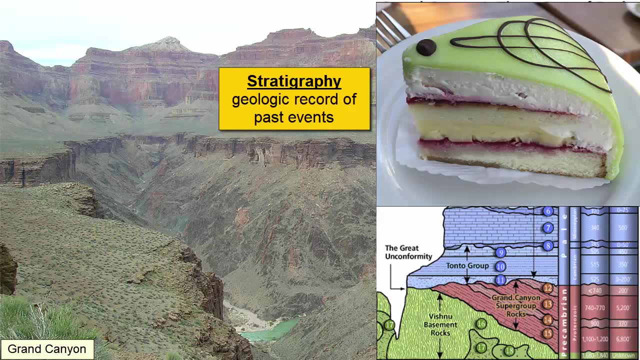 an area, we need to gather as much information as possible, which is helped when we can view the rocks in cross-section, like viewing a slice of cake. edge-on Outcrops at highway, excavations, railroad cuts, stream valleys and cliffs all provide. 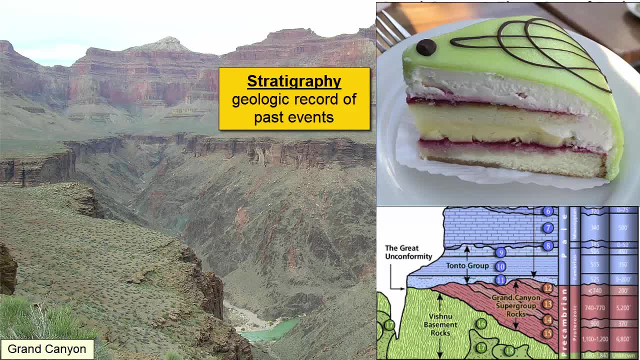 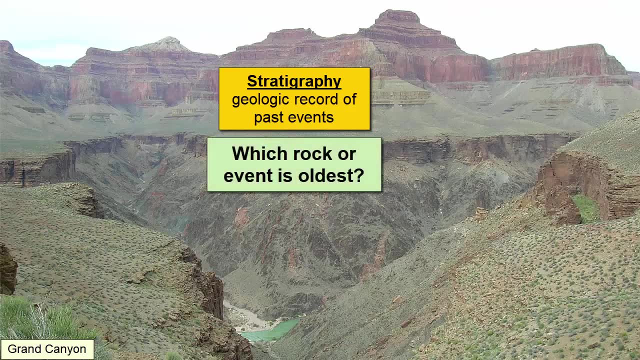 good cross-sections of earth's crust and good libraries filled with information for geologists to interpret. The process of relative dating begins with determining which rocks or event in an area are the oldest. Then each successive event that occurred after that is placed in sequence relative to the 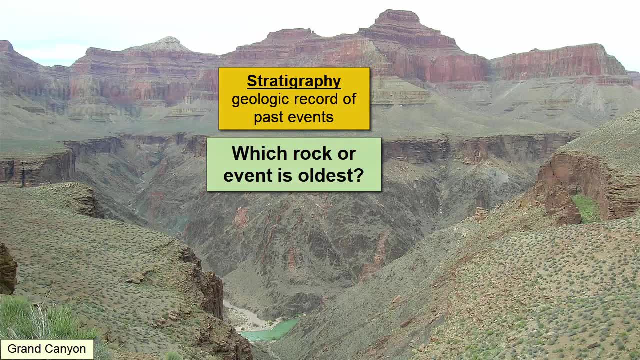 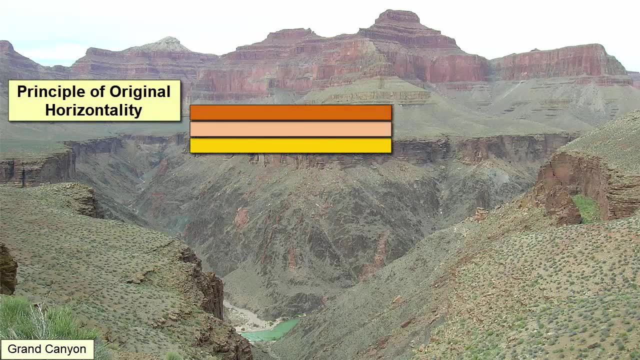 others to build a stratigraphy. The principle of original horizontality describes the general tendency for sediments or lava flows to be deposited or erupted in horizontal layers. The principle of superposition, as already discussed, states that the lowest sedimentary rocks in an undisturbed area are the lowest sedimentary rocks in an undisturbed area. As foroccupation, thechlagen of sedimentary strata is based on the funny thing that the sedimentary strata is the tbspfsequence composite of the sedimentary strata and the 2007 trobos quasar. 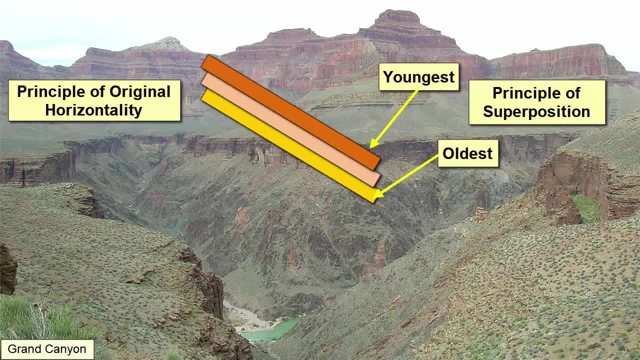 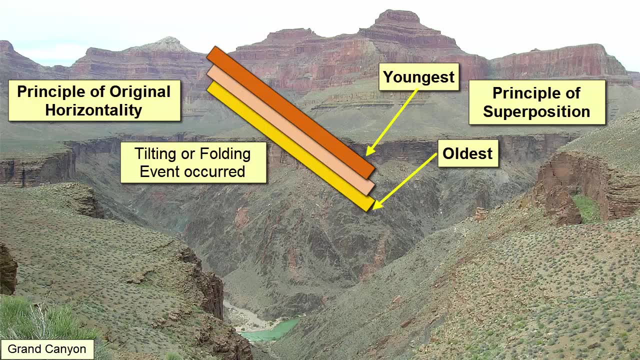 or present-day stratigraphy. These were deposited first and therefore our oldest. If later we see tilted or folded sedimentary strata or lavas, we know that after the original rocks were deposited there was a tectonic event that deformed the layers. 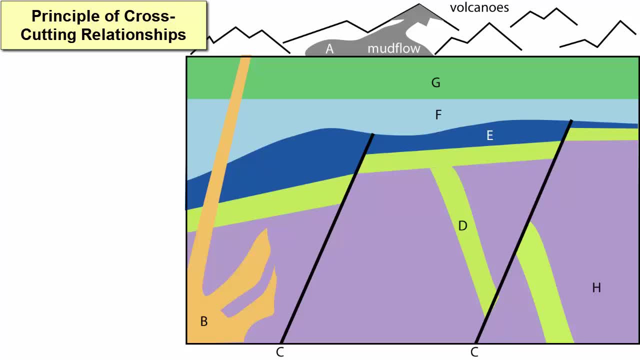 The principle of cross-cutting relationships describes how certain geologic events, such as folding, faulting, magma intrusion and erosion, are younger than the rocks they alter. For example, igneous intrusions are younger than the crustal rocks they alter. The most matrix structures in the geological system are theב. 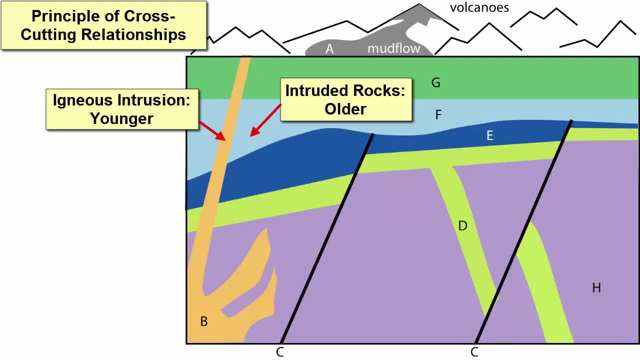 intercutting folding magma, intrusion and erosion. the crustal rock into which they intrude and faults are younger than the strata they fracture. it is often possible to determine the relative ages of several mutually cross-cutting intrusions and faults. inclusions are pieces of one rock that you find in another rock. 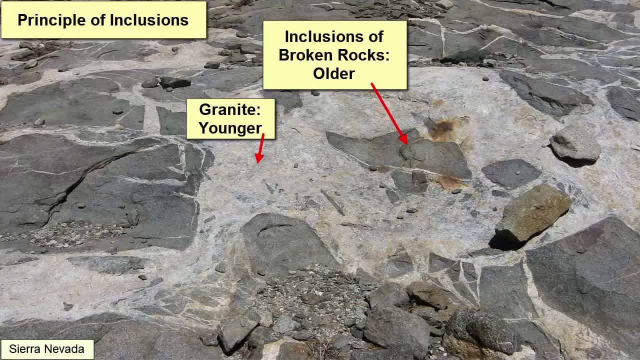 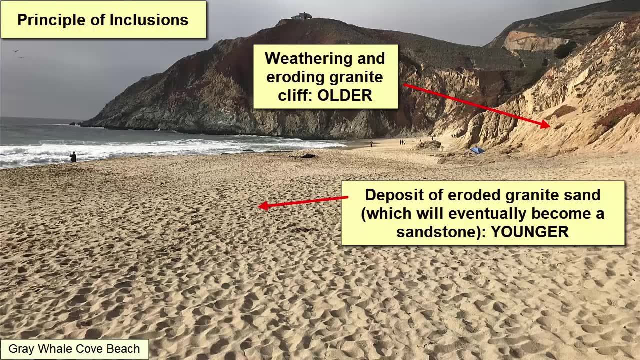 included. rocks must be older than the rocks in which they are found. for example, a cliff face of granite will weather. pieces of the weathered granite will make their way into beach sands. the sandstone that forms from these beach sands must be younger than the granite pieces within. 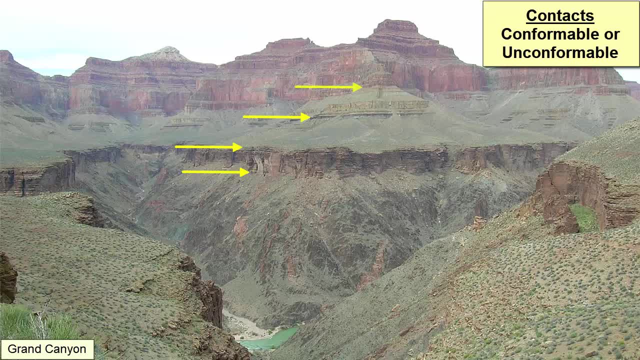 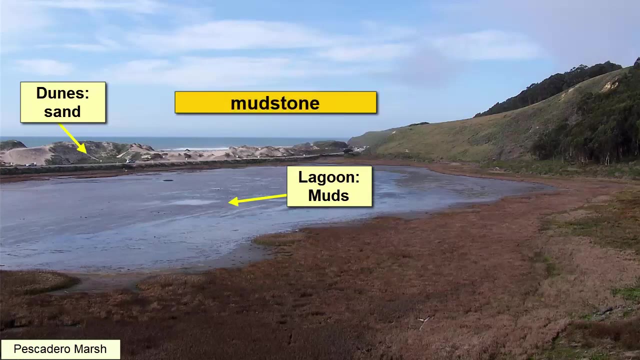 let's look more closely at the contacts between rock layers. what do they represent? usually these are conformable, meaning that rocks on both sides of the contact formed at about the same time, but in between the environment changed. for example, a mudstone might represent muds depositing in a. 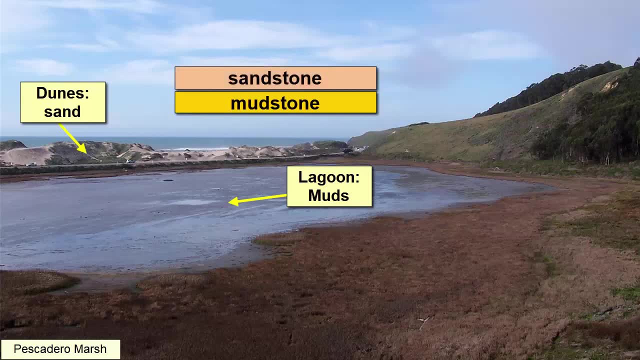 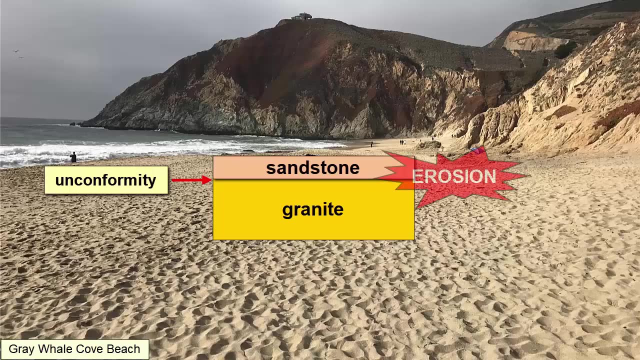 lagoon, but eventually nearby sand dunes migrate and cover up the lagoon, so sands will deposit on top of the muds through a shift in the environmental conditions. an unconformity is a contact between two layers that represents a pause in deposition in an area. 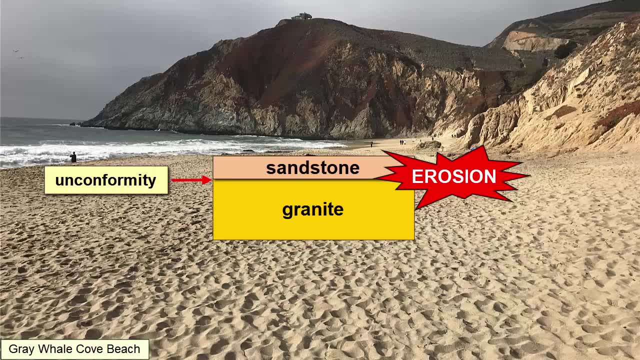 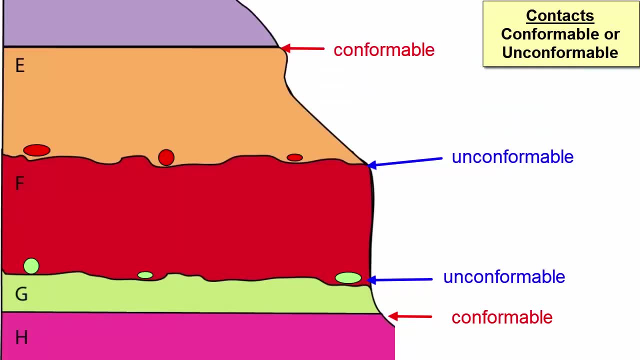 or when an area has been uplifted and eroded. how can we tell which kind of contact we're looking at- conformable or unconformable? when we look carefully at the contact, if we see evidence of erosion, such as an irregular surface, excavation or inclusions of the rocks below the contact, it's 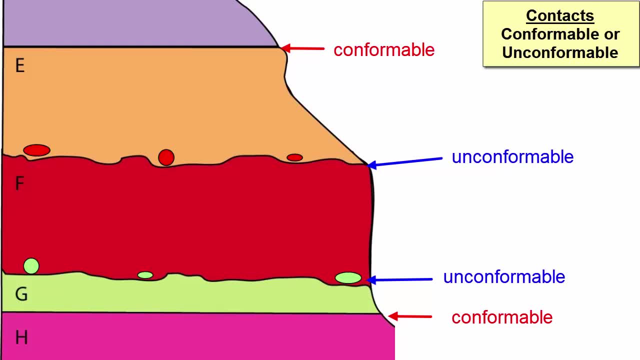 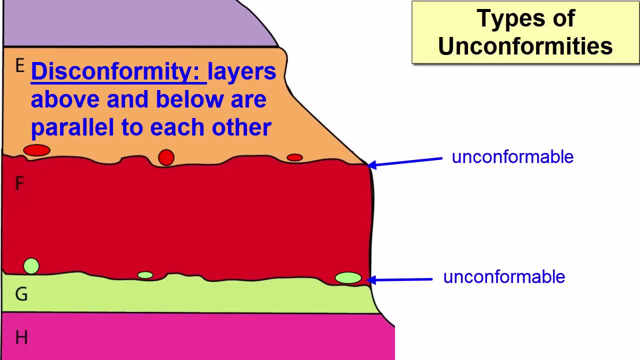 not always the case that there is erosion at work between the layers above the contact. we know there was erosion at work before that layer above was deposited. we can further divide unconformities by their type to provide us with more information about the events that took place in a particular area. disconformities are unconformities between: 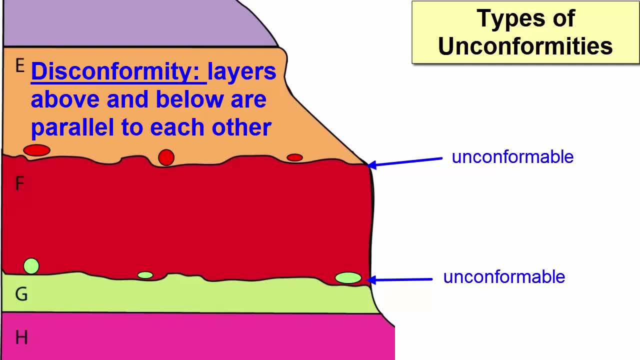 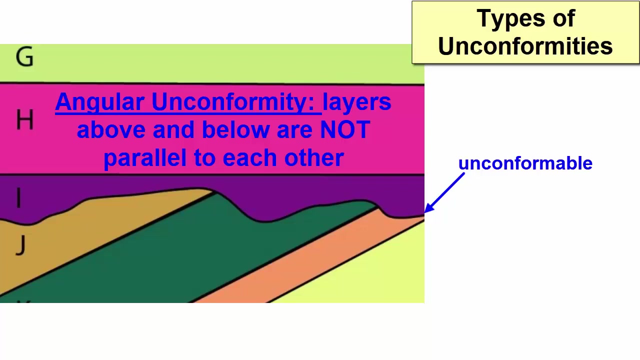 parallel strata or lava flows. usually the contact is irregular and pieces of the underlying rock are included in the strata above. these unconformities indicate erosion or a small time with no deposition but no tectonic transformation and no excavation to deeply buried rocks. angular and conformities are unconformities where the parallel sedimentary layers or lava flows. 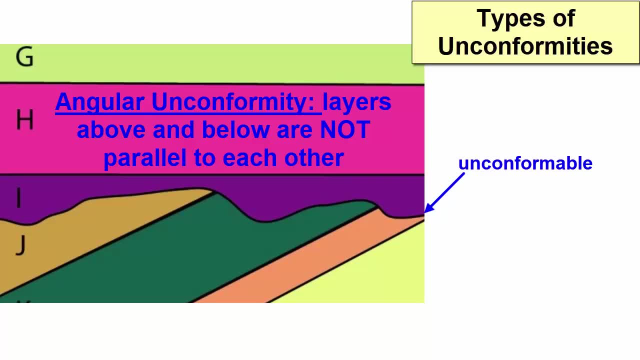 above the contact are at an angle to the parallel sedimentary layers or lava flows below to see an angular and conformity in an area means the area was subjected to tectonic activity that caused folding or tilting before erosion and renewed deposition non-conformity. 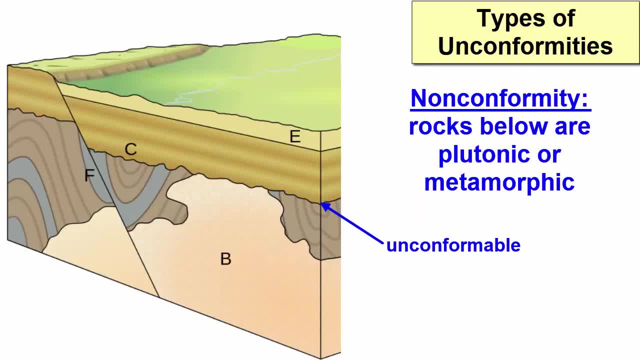 these are unconformities with intrusive igneous rock or metamorphic rock below and parallel sedimentary rock layers or lava flows above the layers on top which would have formed originally on our surface. sit atop uplifted and eroded igneous or metamorphic rock that formed 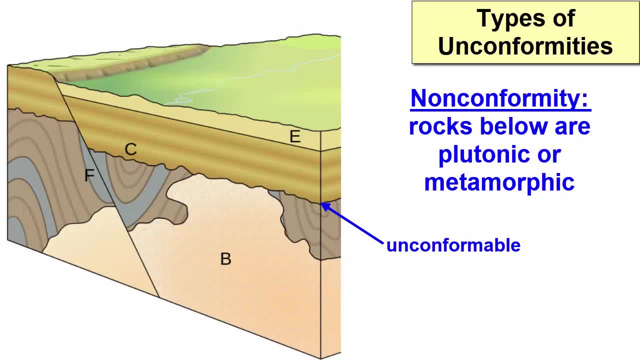 originally at depth. that means those deep rocks were exposed at one point on the surface. to bring deep rocks to the surface requires significant uplift in erosion and the loss of many layers of rock, many missing books in our surface surface. surface rock is a very important part of our 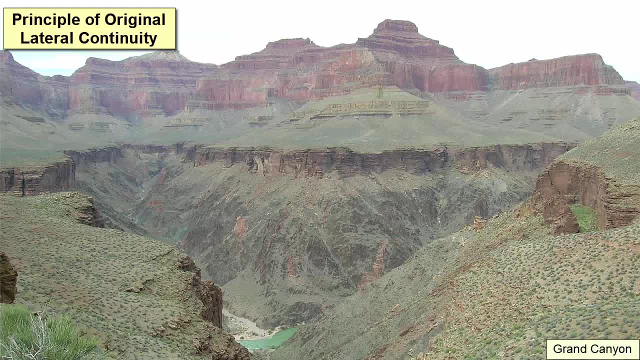 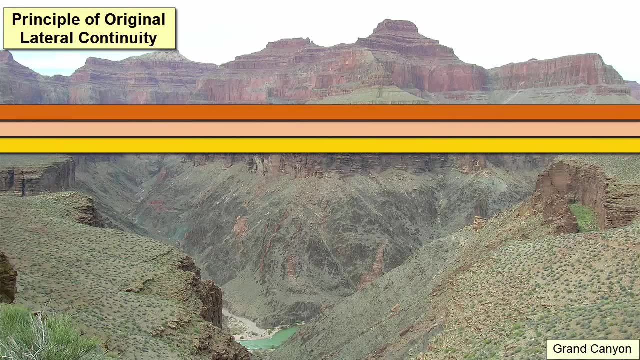 environment, and it is a very important part of our environment and it is a very important part of our geologic history. the principle of original lateral continuity describes the tendency for lava flows and sedimentary beds to extend laterally in all directions until they thin to nothing. 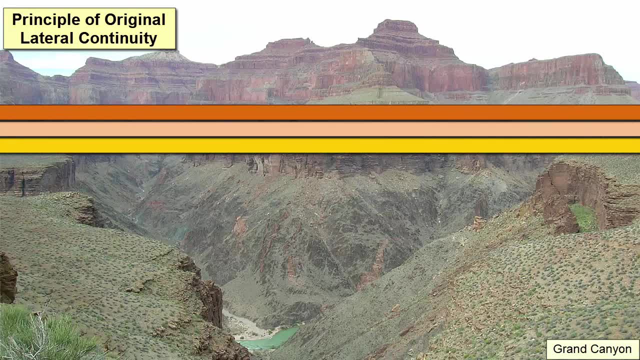 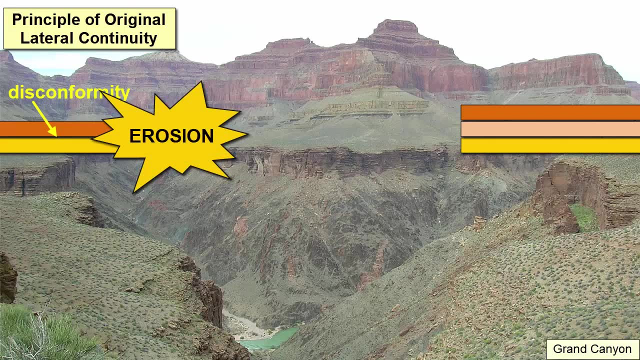 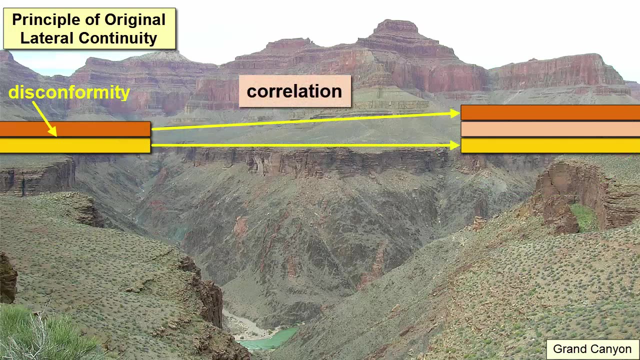 or reach the edge of the depositional basin. in other words, they don't simply disappear. so if we have an unconformity in our local stratigraphy and one or a number of rock layers have been eroded, we can look around to surrounding areas if we can correlate the layers above and below the unconformity. 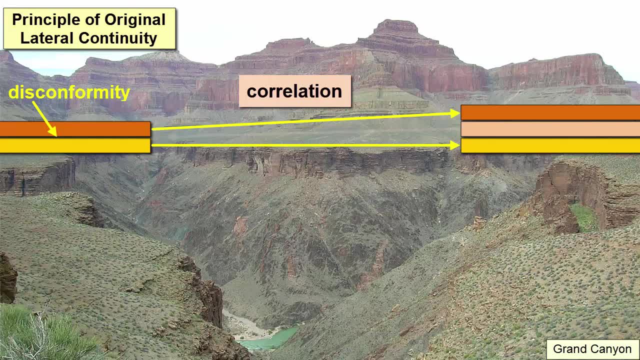 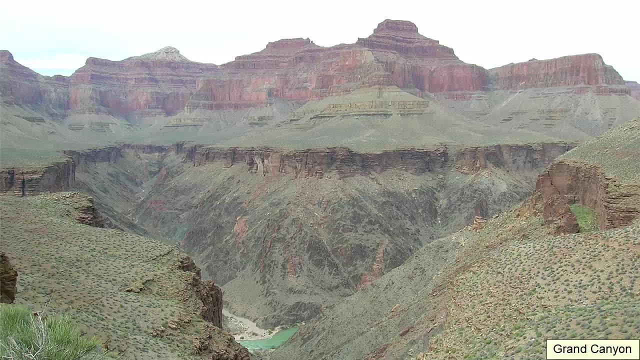 with those same layers elsewhere. we can use the intervening rocks in the surrounding area to fill in the gaps that might exist. in our local story we call that process correlation. let's practice these principles by building a stratigraphy for a cross-section through the grand canyon. if you were to hike down into the grand canyon, here's the top where you would start. 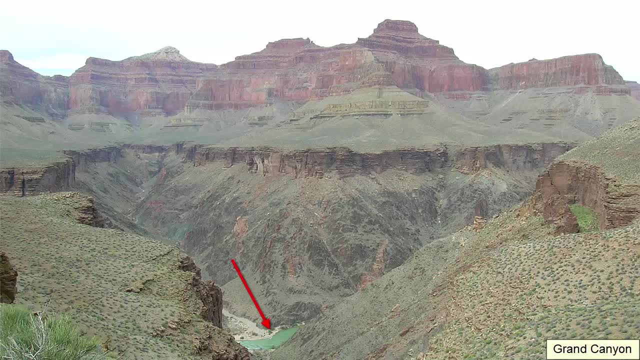 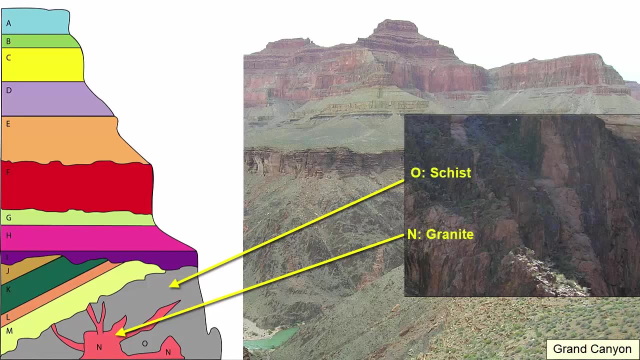 and here's the base where the colorado river runs. where is the oldest rock? the ones that appear closest to the bottom? the ones that appear closest to the bottom. the ones that appear closest to the bottom are: o a schist and n a granite. we know that granites intrude into existing rocks. 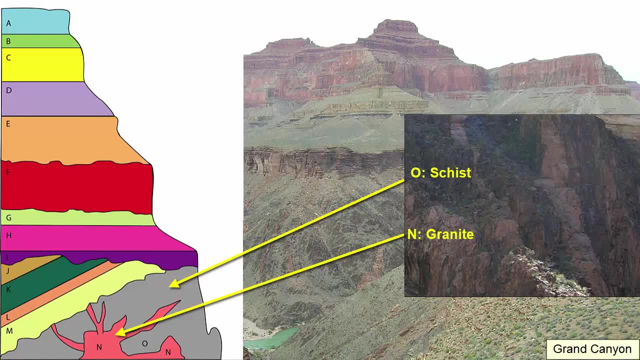 so unless that granite has signs of being exposed at the surface and eroding, the schist likely happened first, also schist formed through high-grade metamorphism. and if the granite had been inside the schist before or as it was metamorphosing, the granite would have also 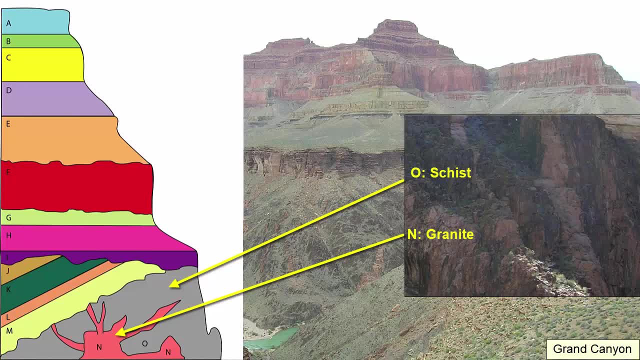 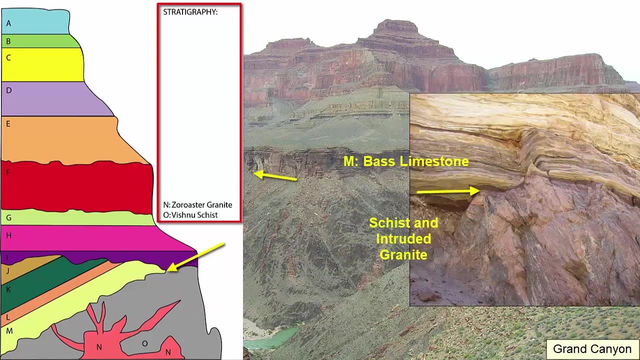 turned into a schist. so all these clues, plus the shape of the intruding granite, tell us that the schist was there first and is thus the oldest, followed by intrusion of the granite. we now have the first two events at the base of our stratigraphy determined what next we see a 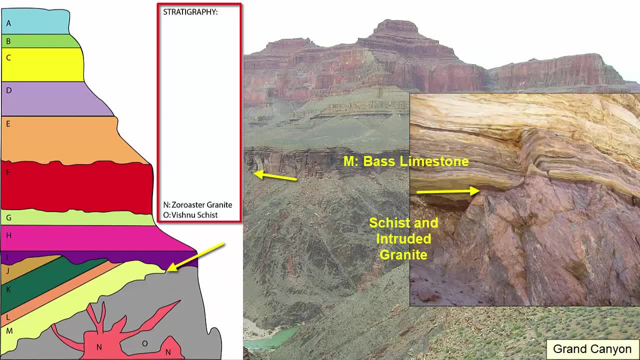 contact that looks irregular between the schist and granite and the bass limestone m which sits above. based on the irregularity of the surface and the fact that granites and schists form deep underground while limestones form on the surface, we can label this contact as a non-conformity. 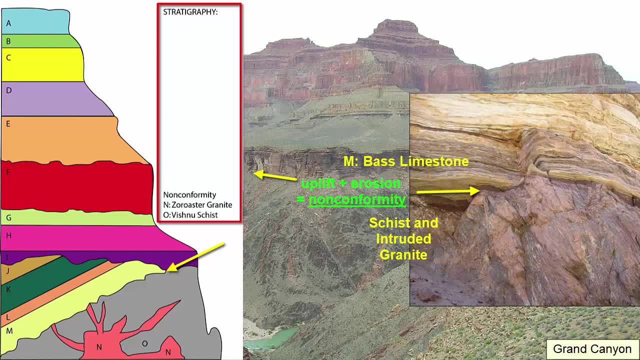 schist and granite when they formed, but those layers have since been removed through erosion. therefore, we have erosion happening potentially over many millions of years and then, after the erosion stops, likely because the area has been eroded. flat deposition resumes and m is laid down, followed by l, k and j. 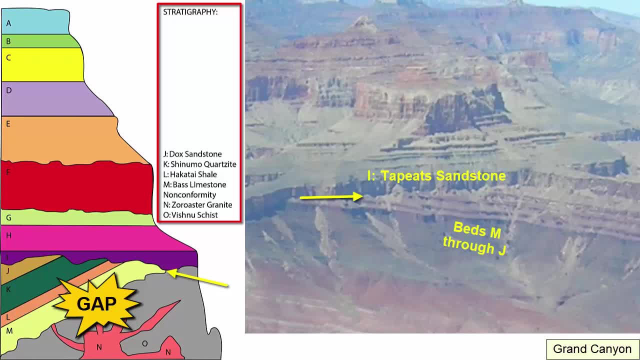 the contact between j and the rocks above i is also irregular, indicating erosion. furthermore, the rocks below the contact are in an angle to the ones above. here is where we see evidence of a tectonic event that tilted the rocks, after which the area was eroded flat and deposition began. 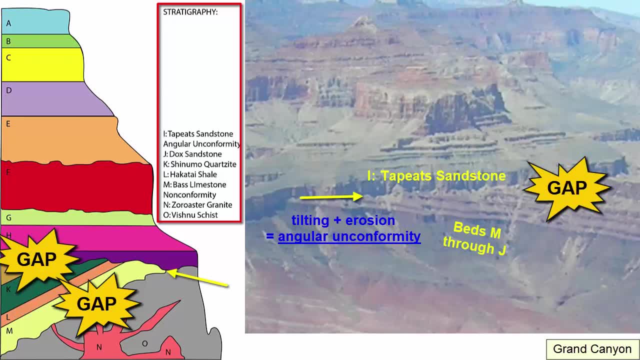 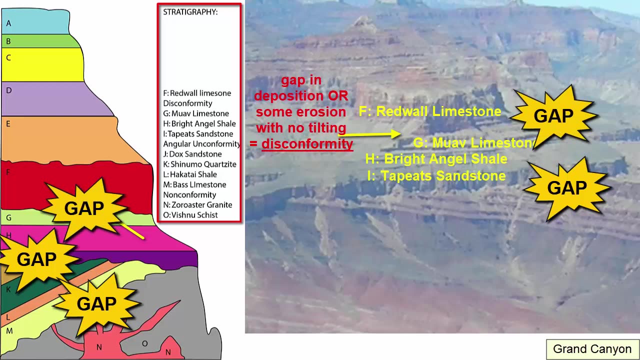 again with i. so between j and i we have an angular unconformity. after i was laid down, h was laid down, followed by g. then between g and f we see an irregular eroded surface, which is a disconformity, as there's no tilting happening prior to erosion. 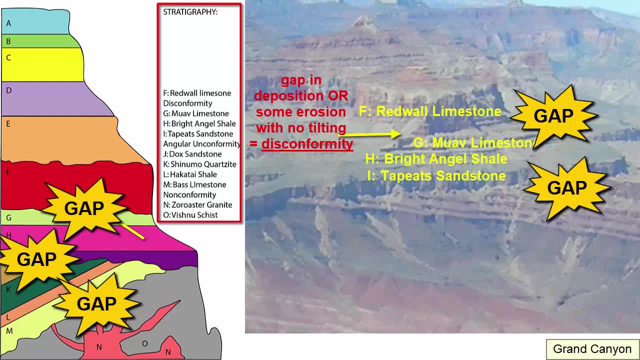 immediately below the surface aren't deep metamorphic or plutonic igneous rocks. After the erosional event, F is laid down and then again a disconformity appears. That means we don't know how many other rocks had been laid down after G and before F, or after F and before the rock above. These are gaps in. 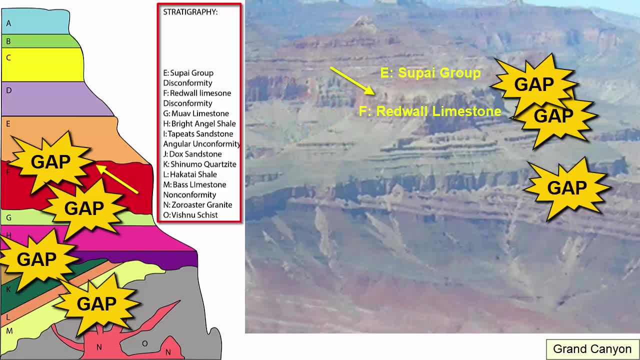 our story. After the erosion to F, deposition resumes and we see bed E laid down, followed by D, C, B and A. We don't know how many more rocks were laid down after A, because the area is currently experiencing erosion by the Colorado River and the top of A is an eroded 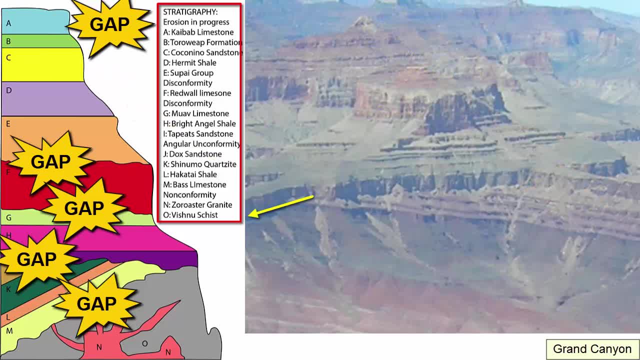 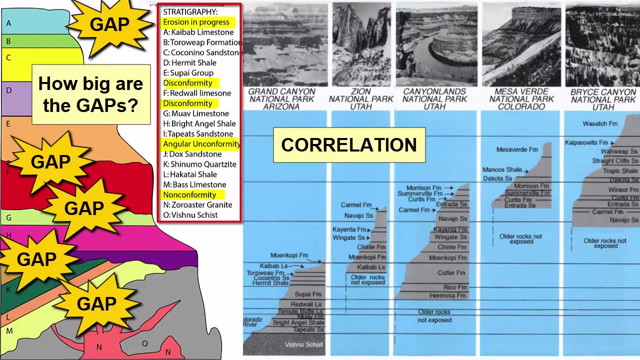 surface. This vertical timeline with oldest on the bottom and youngest on the top, is our complete stratigraphy. Gaps in our story exist everywhere. there's an unconformity. How much of a gap To determine that we could try to correlate with surrounding geology, which it turns out is possible with the nearby Bryce? 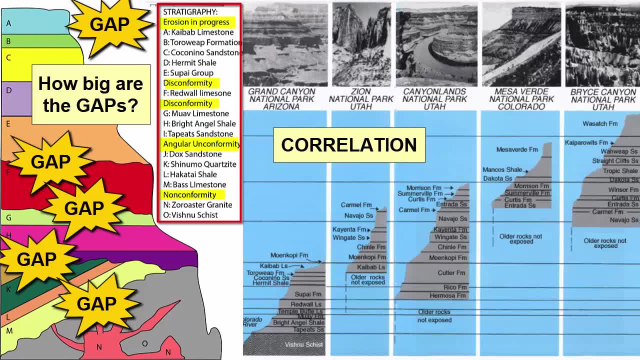 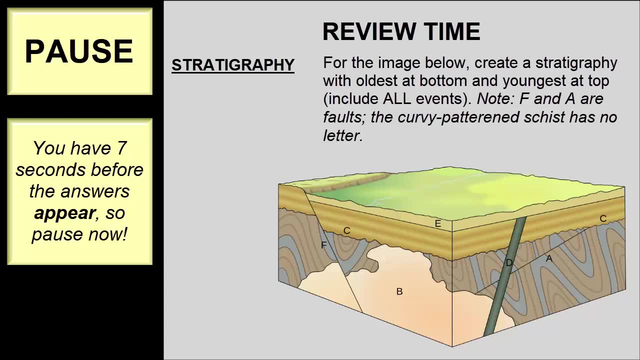 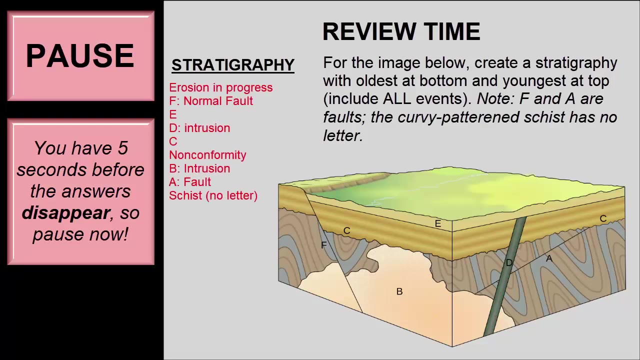 Canyon and Zion National Parks. We could also conduct numeric dating on the rocks above and below if they contain the right ingredients for radiometric dating. Or we can use fossils. Pause now. Fossils are direct or indirect evidence that a particular organism lived in an 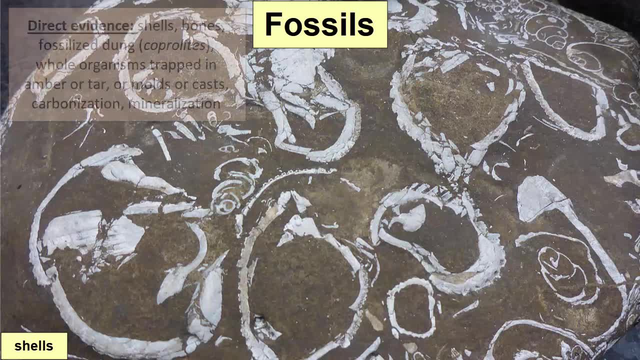 area at the time the rock was formed. Direct evidence would be that the rock has been buried in the rock for a long period of time and that the rock has been buried in the rock for a long period of time and that the rock has been 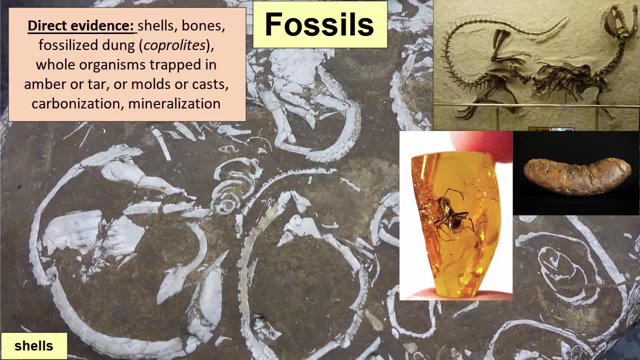 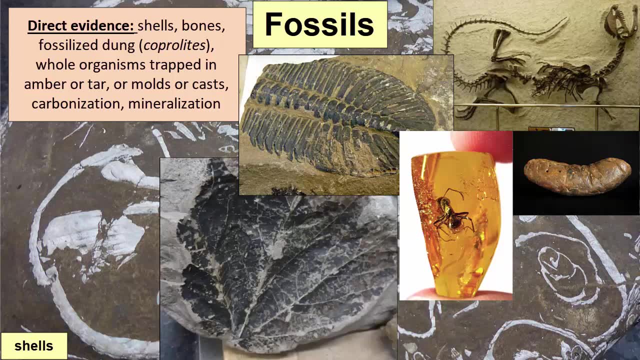 buried in the rock for a long period of time. Fossils would be shells, bones, fossilized dung, known as coprolites, whole organisms trapped in amber or tar, or molds or casts of the organism. Sometimes organisms like leaves will leave a carbon film on the surface of rocks after. 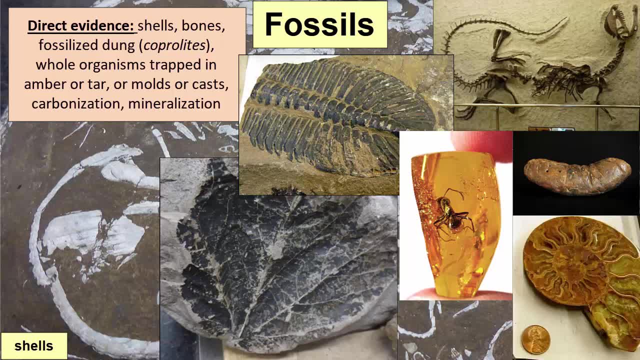 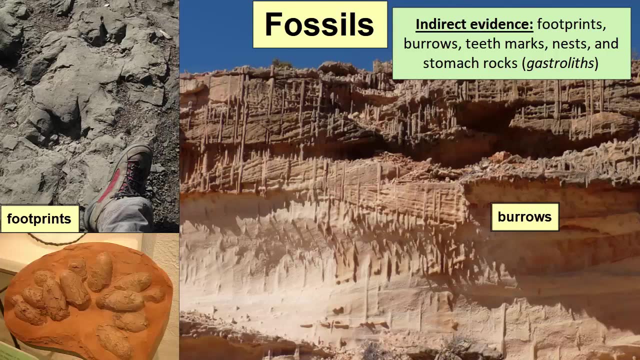 they've been buried and broken down. Sometimes the original buried shells will be replaced by minerals. In all these cases, the evidence we find is some part or all of the organism's body. Indirect fossil evidence includes footprints, burrows, teeth marks, nests and stomach rocks known as gastroliths- Evidence that an 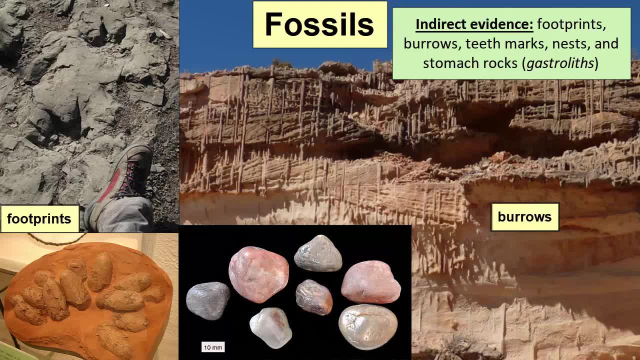 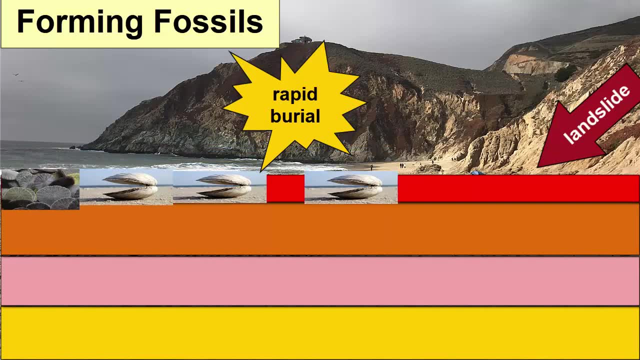 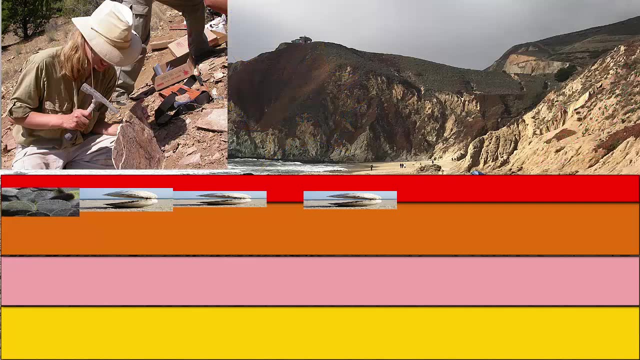 organism was in the area, but very little about its structural shape. To form any of these fossils, we first have to rapidly bury the dead organism or its indirect mark, and thus preserve it in rock layers at depth. Paleontologists study the evolution of Earth's life through the study of fossils. 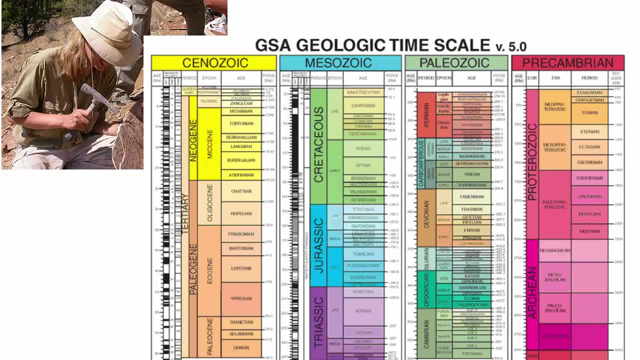 They have collectively created the geologic timescale which breaks Earth history by the size of the Earth's surface. They have collectively created the geologic timescale which breaks Earth's history by the size of the Earth's surface. they have collectively created the geologic timescale which breaks Earth's surface. 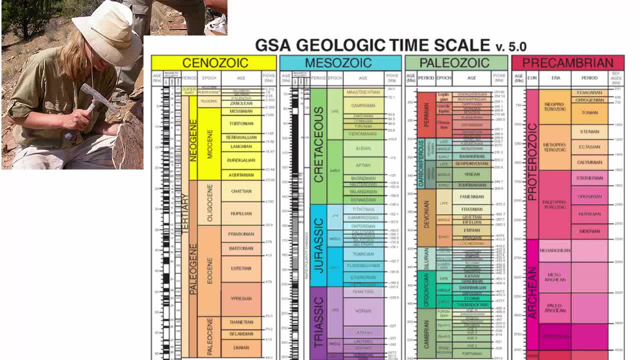 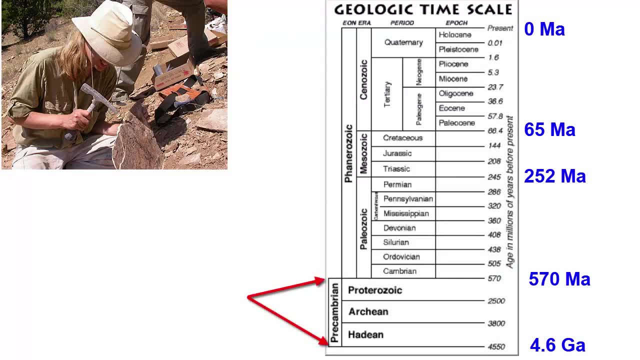 into particular eons, eras and periods, each given its own name, based on rocks studied from that period somewhere on the planet. studied from that period somewhere on the planet, According to this time scale, the first four billion years of Earth's history. 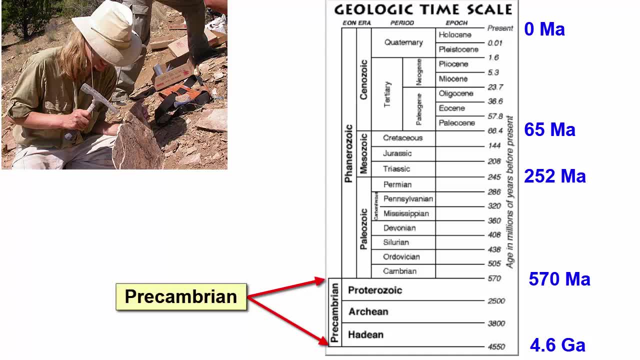 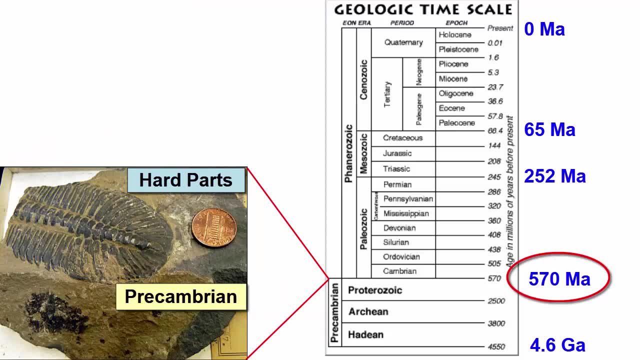 According to this time scale, the first four billion years of Earth's history is collectively known as the Precambrian. Why that date? for The Boundary, The oldest fossil evidence we have of organisms that have hard parts. After hard parts were developed by living organisms, it was easier to preserve them. 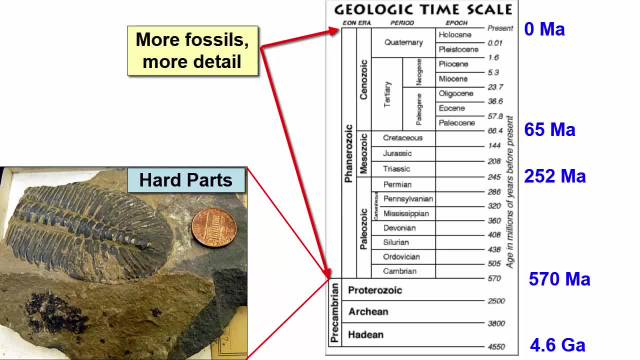 as fossils when they died. therefore, much more fossile evidence, fossil evidence available to differentiate different events and environments in Earth's history, Especially extinction events. Paleozoic, Mesozoic and Cenozoic are each separated by major extinction events on the planet, the largest of which. 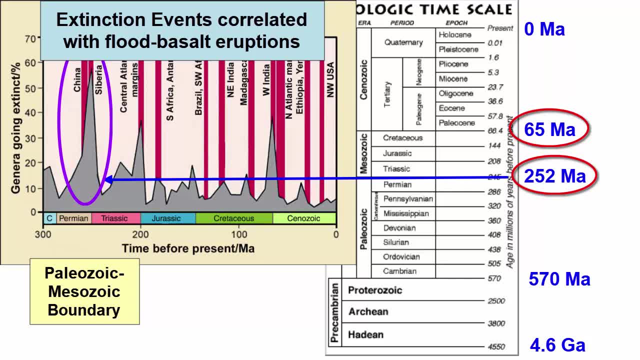 happened at the end of the Paleozoic, 252 million years ago, known as the Permian extinction. What caused this extinction? Likely the eruption of a new hotspot and the pouring out of the Siberian Trap flood basalts. The end of the Mesozoic is 65 million years ago, also known as the Cretaceous-Tertiary. 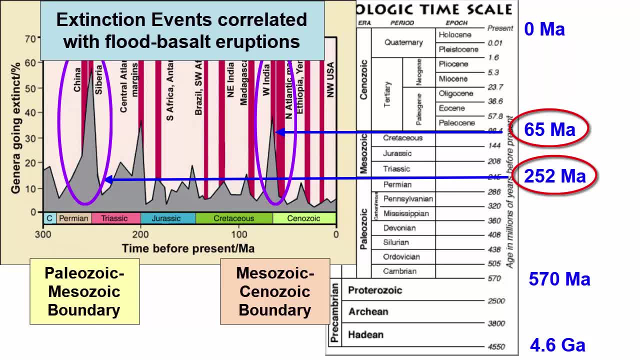 boundary or K-T boundary. It corresponds to another major extinction event, this one involving the extinction of all dinosaur species. The cause of that extinction was likely the eruption of the Deccan Trap's flood, basalt province, combined with a large asteroid hit. 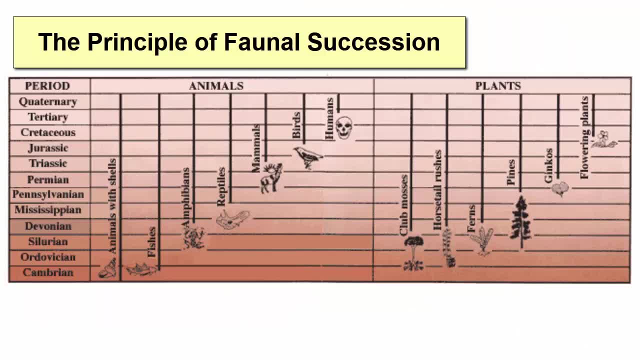 The principle of faunal succession. The principle of faunal succession describes how flora and fauna succeed each other in a reliable order based on evolution and extinction. We can use fossils of these organisms, therefore, to assist with relative dating and, in particular, to help us determine the extent of gaps for our unconformities. 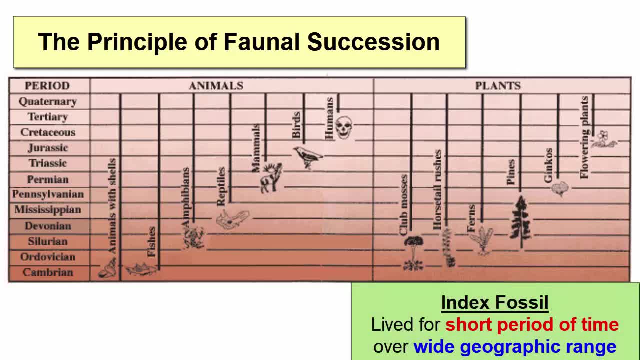 Fossils of organisms that live for very short periods of time across a wide habitat geographically are called index fossils. We can use them to better narrow the possible ages of a rock and to correlate rocks from one part of the world with those of another. 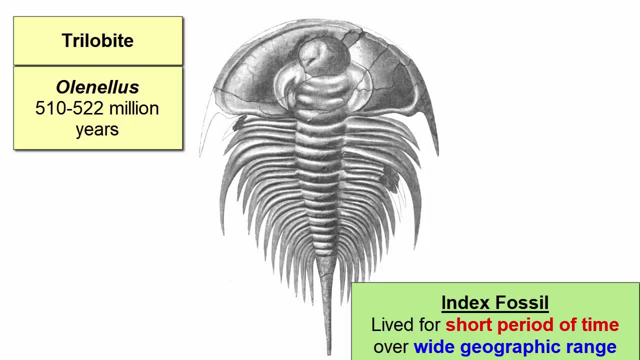 The genus Solanellus is a great example of an index fossil, as these marine organisms lived across the world's oceans between 510 and 522 million years ago. Stromatolites, on the other hand, are marine organisms that have existed on planet Earth. 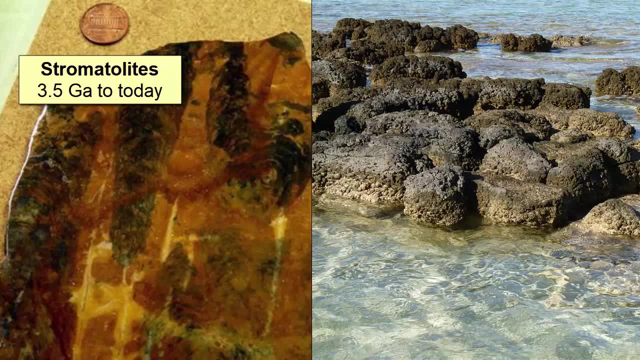 for the last 3.5 billion years? What do we know if we find a fossil stromatolite in a rock That its age is between today and 3.5 billion years ago? Not so useful in terms of relative dating.